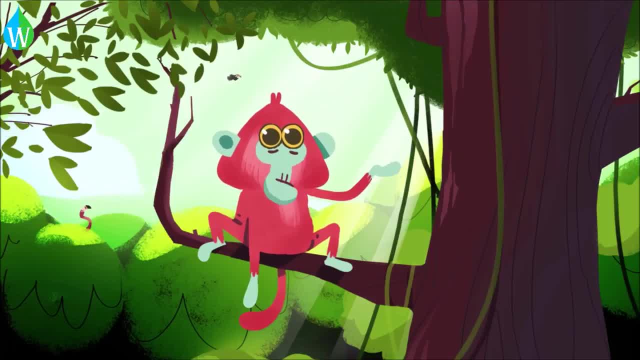 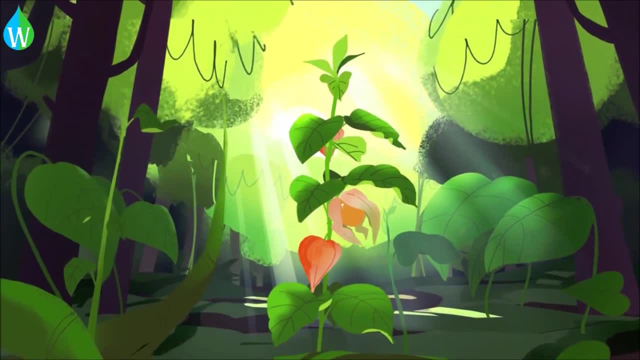 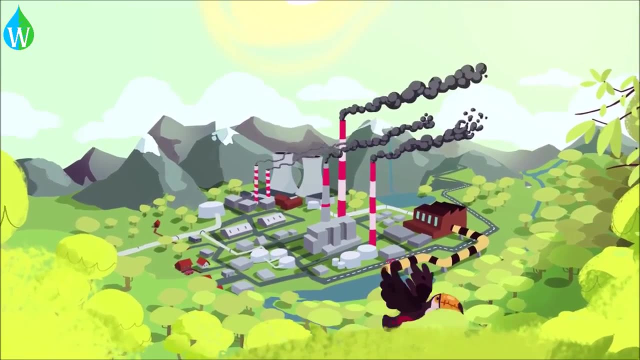 We have many natural ecosystems that must be in balance in order for us to live here. The climate system is one of them. This system ensures that the temperature is correct and that the atmosphere emits exactly the right amount of solar energy. When we emit harmful greenhouse gases such as CO2,, we clog the atmosphere. 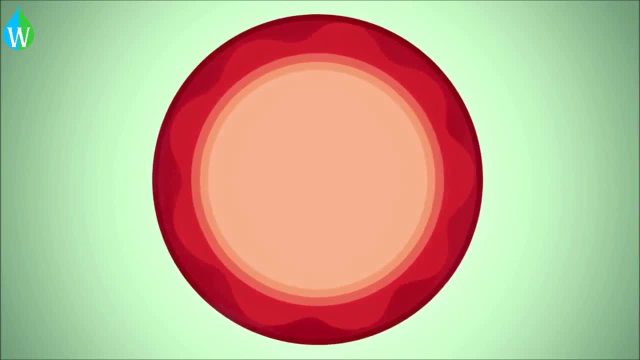 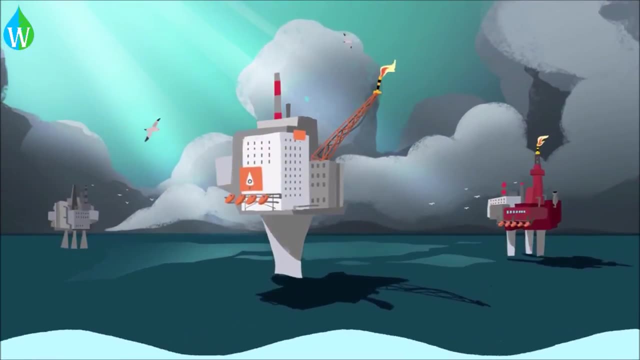 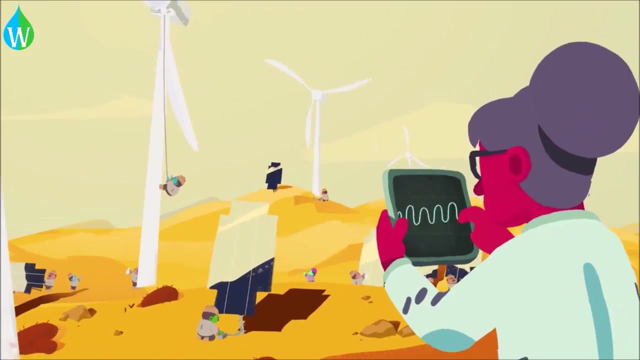 This changes the temperatures on Earth, which again affects our development. How we produce and use energy is incredibly important. Oil and coal are examples of energy. we may run out of Water, wind and sun. however, will always be here, Using the lasting sources of energy that renew themselves. 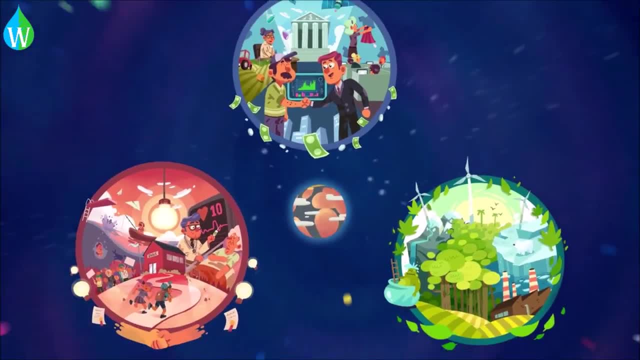 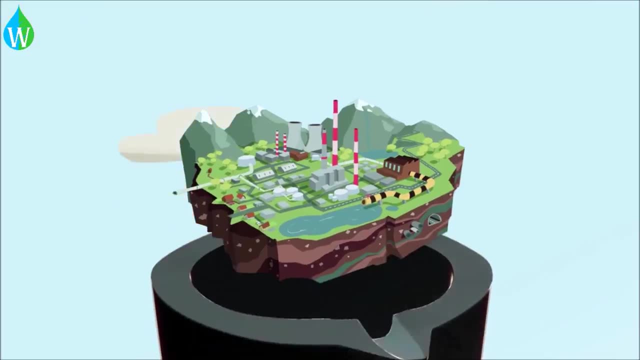 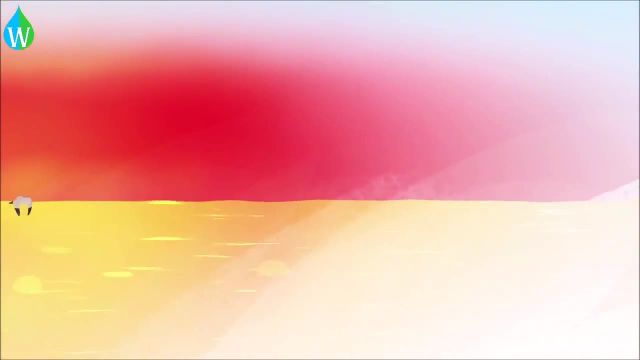 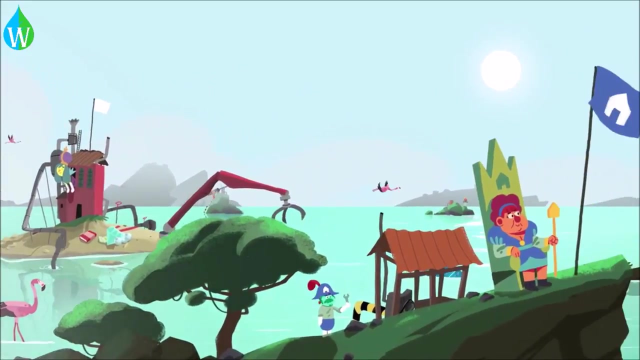 is good for the planet and can provide jobs for years to come. Economics: Almost everything we develop, buy and trade starts with nature. The smarter we use our natural resources and the better systems we create for a fair distribution, the more sustainable we are. 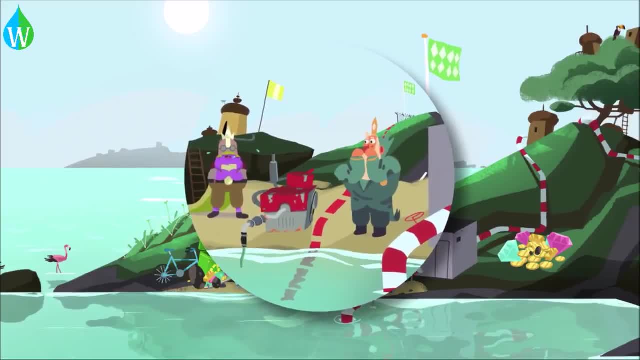 One way to contribute to the environment is to use natural resources. One way to contribute to the environment is to use natural resources. One way to contribute to the environment is to use natural resources. To give nature an equal distribution is to be more aware of what we buy. 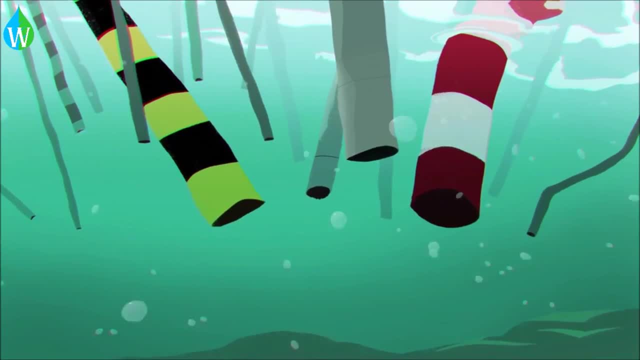 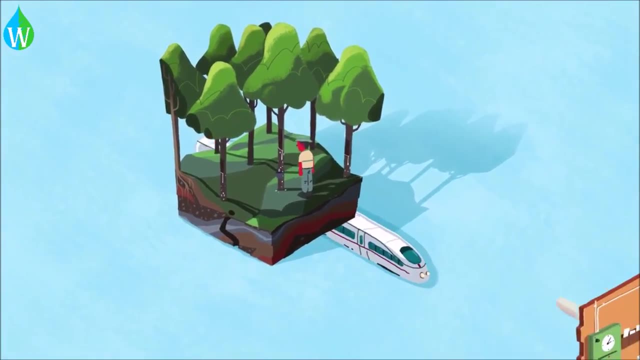 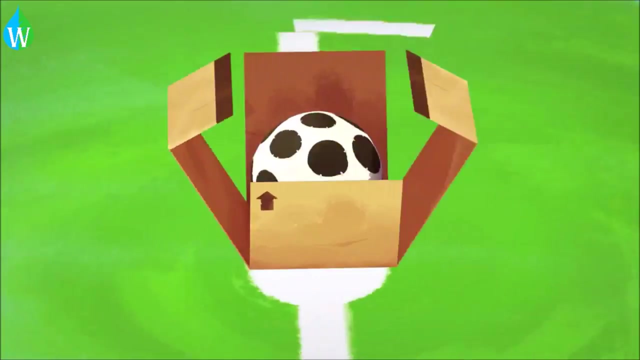 and how it is produced. A football is a good example. It travels far before it reaches the football players. First the materials are made, Then they print the logo somewhere else before a third country sees it all together. One single football sees the whole world before it reaches its goal. 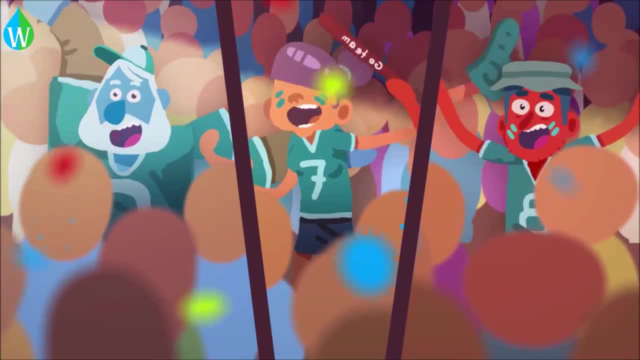 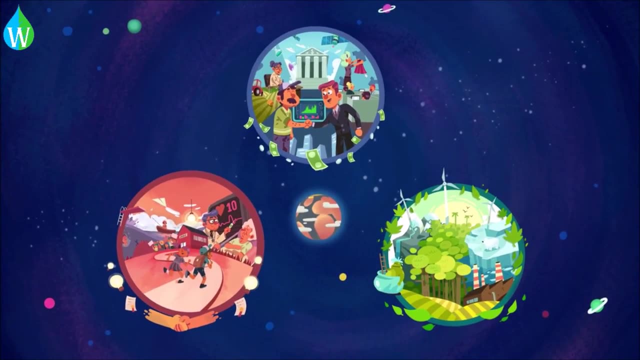 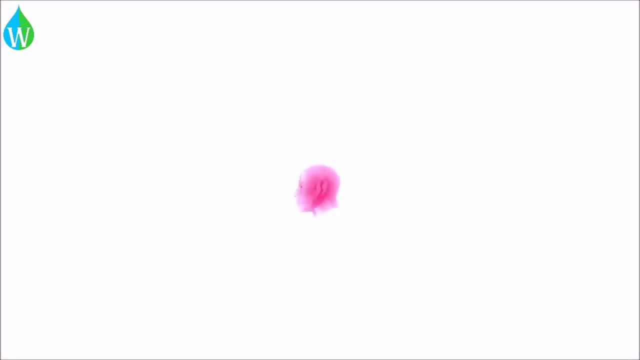 This journey ties us together. This journey ties us together: win the battle for a sustainable future. we have to play with fair rules. that applies to everyone: social progress. we humans are part of nature, but we're also important resources for the world, just like water, the forest and the sun. we have minds that can create the strangest and most. 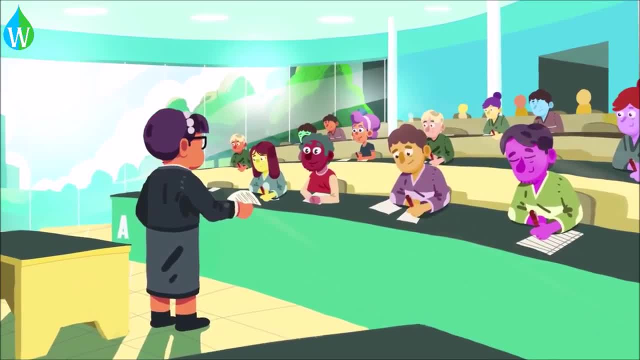 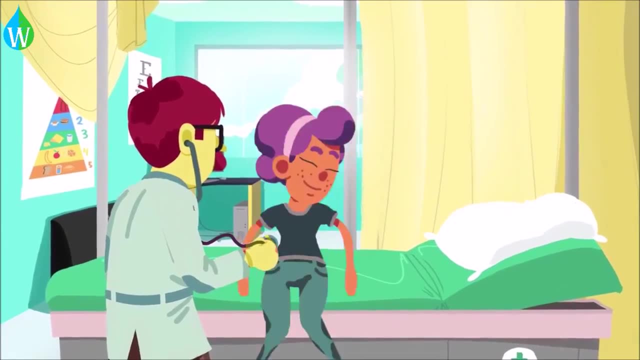 creative things, but for us to be the best versions of ourselves, there are certain things that must be in order, like having equal opportunities to education, safety, food and medicine. this provides greater opportunities for us as human beings, but also for the planet. we just have to think in new.